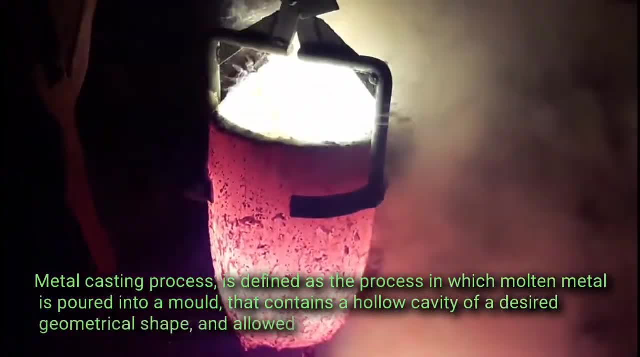 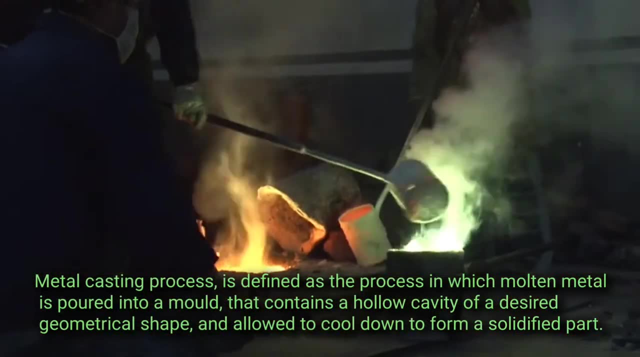 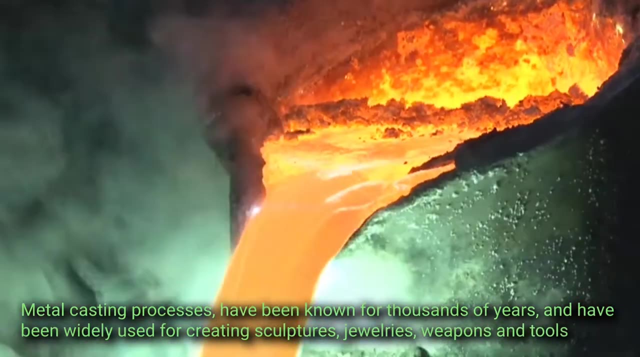 Metal casting process is defined as the process in which molten metal is poured into a mold that contains a hollow cavity of a desired geometrical shape and allowed to cool down to form a solidified part. Metal casting processes have been known for thousands of years and have been widely used. 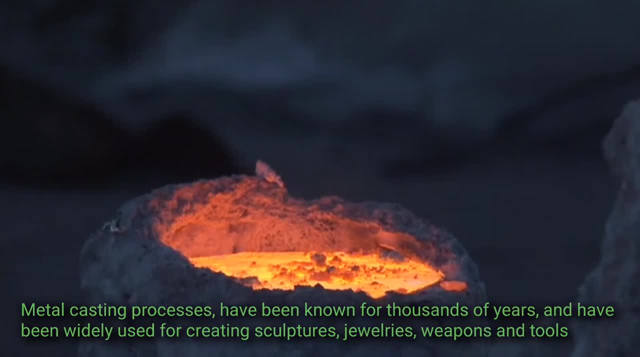 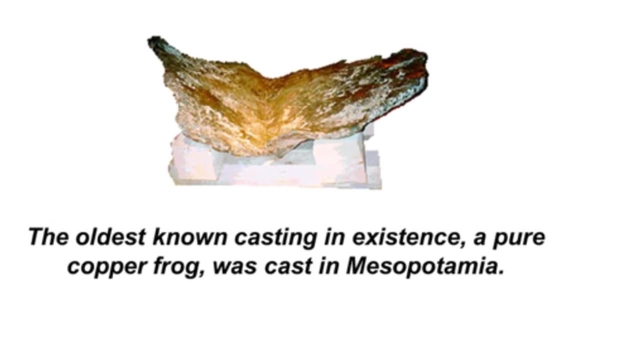 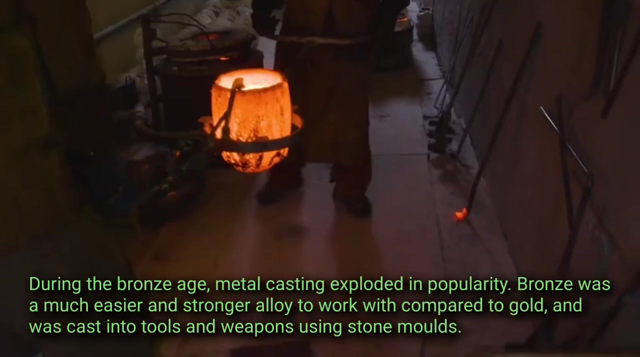 for creating sculptures, jewelries, weapons and tools. The first known cast object is a copper frog that dates back to 3200 BC, found in Mesopotamia, present-day Iraq. During the Bronze Age, metal casting exploded in popularity. Bronze was a much easier and stronger. 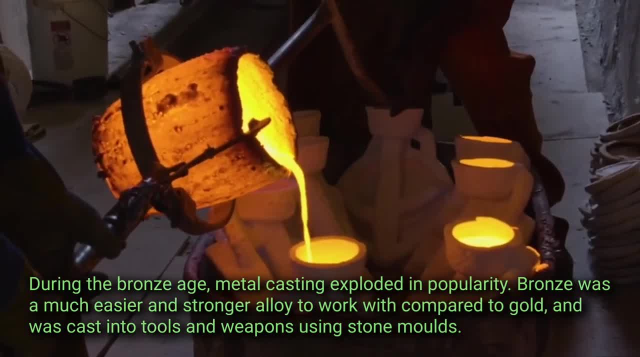 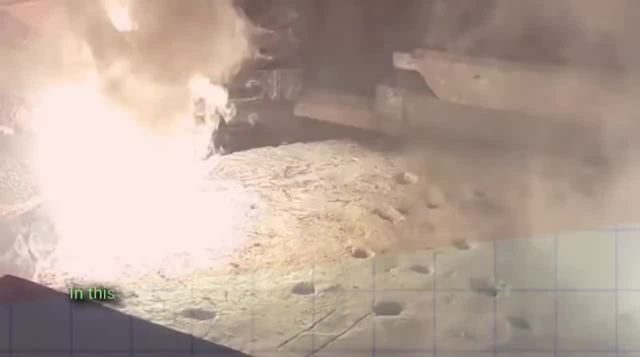 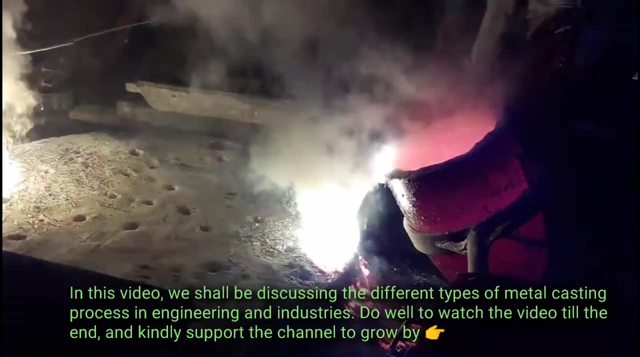 alloy to work with compared to gold, and was cast into tools and weapons using stone molds. Welcome to James Sword Research Channel. in this video we shall be discussing the different types of metal casting process in engineering and industries. Do well to watch the video till the end. kindly support the channel to grow by subscribing to it. 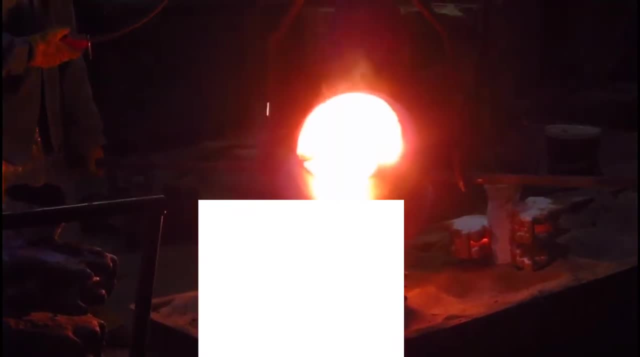 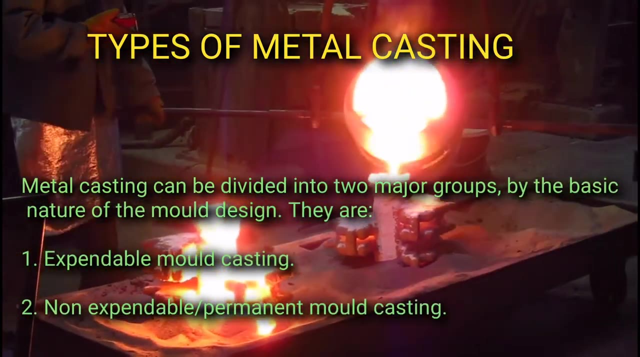 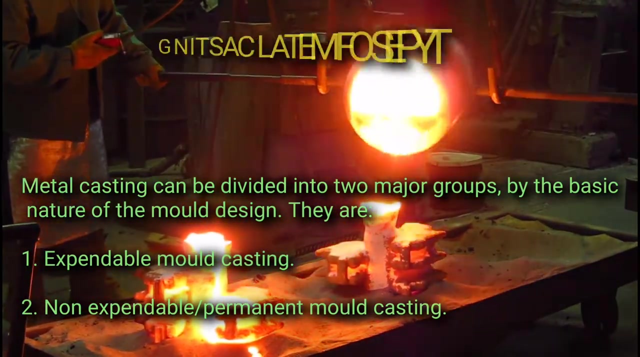 if you're new here and also turn on notification for new uploads. Metal casting process. Types of Metal Casting. Metal casting can be divided into two major groups by the basic nature of the mold design. They are: 1. Expendable mold casting. 2. Non-Expendable or permanent mold casting. 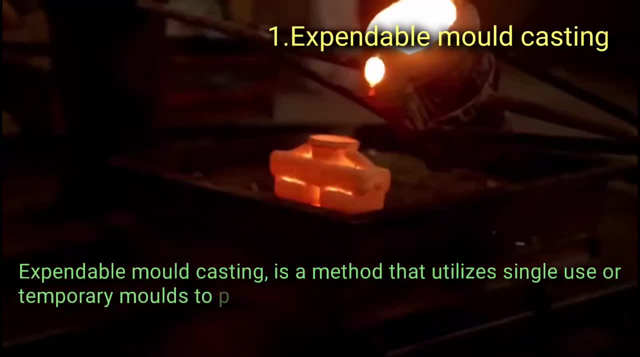 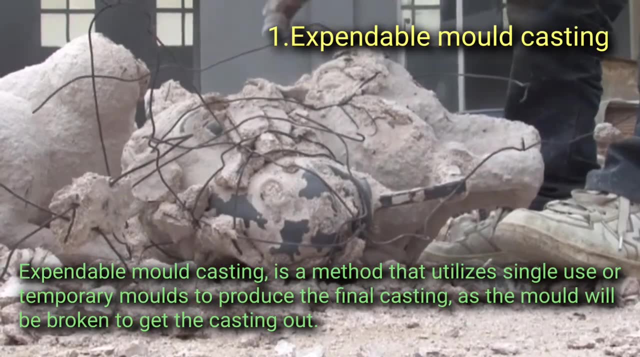 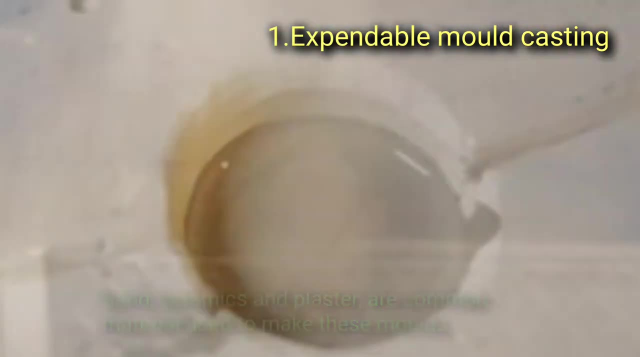 Expendable mold casting. Expendable mold casting is a method that utilizes single-use or temporary molds to produce the final casting, as the mold will be broken to get the casting out. Sand, ceramics and plaster are common materials used to make these molds. They are generally bounded using binders. 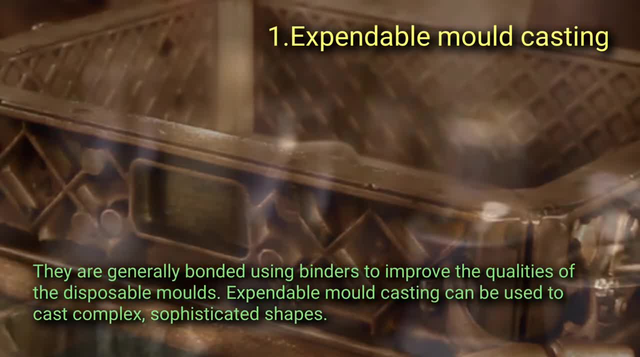 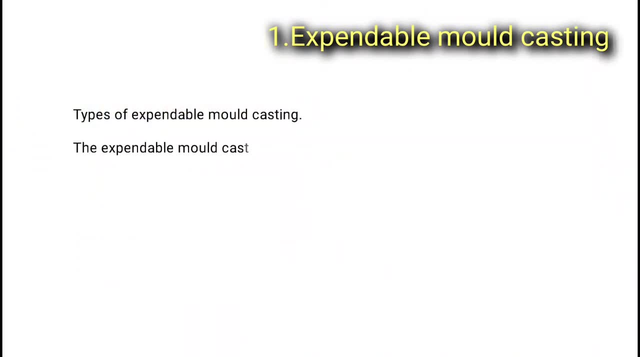 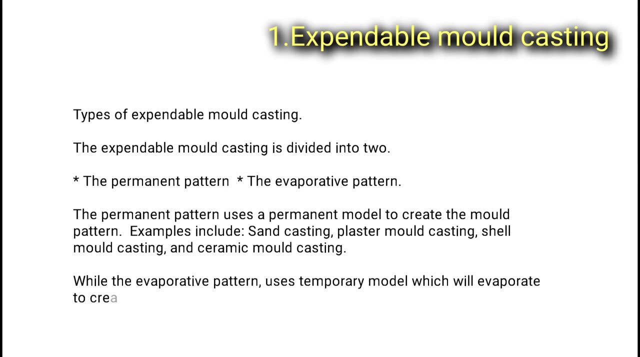 to improve the qualities of disposable molds. Expendable mold casting can be used to cast complex, sophisticated shapes. Types of Expendable mold casting. The expendable mold casting is divided into two: the permanent pattern and the evaporative pattern. 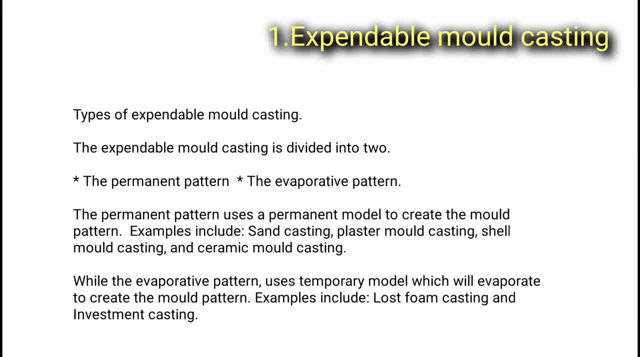 The permanent pattern uses a permanent model to create the mold pattern. Examples includes sand casting, plaster mold casting, shell mold casting and ceramic mold casting, While evaporative pattern uses temporary model which will evaporate to create the mold pattern. Example includes: 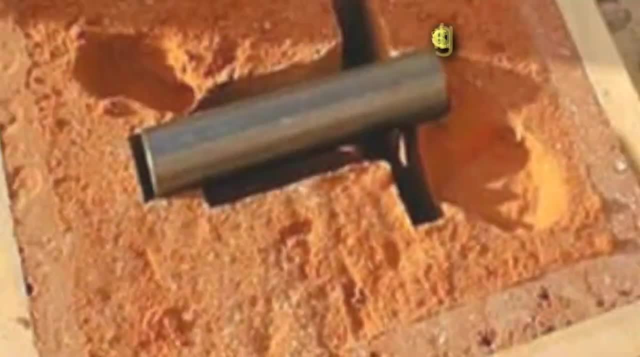 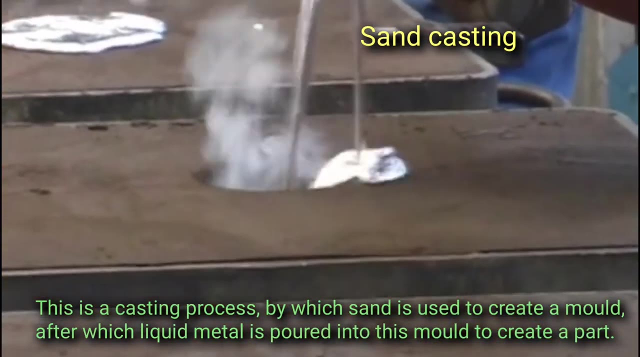 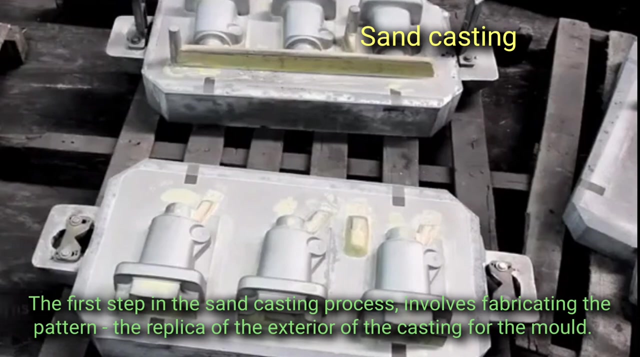 lost. foam casting and investment casting. Sand casting: This is a casting process by which sand is used to create a mold, after which liquid metal is poured into this mold to create a part. The first step in the sand casting process involves fabricating the pattern, the replica of the exterior of the casting for the mold. These 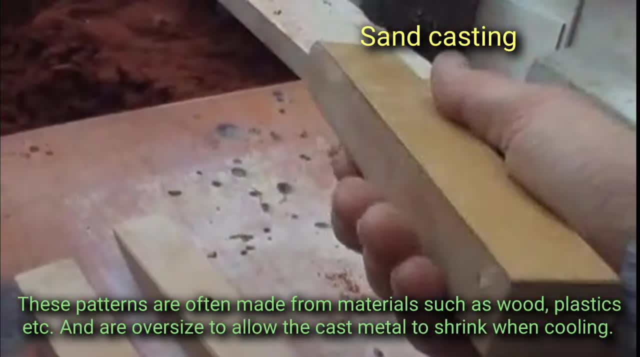 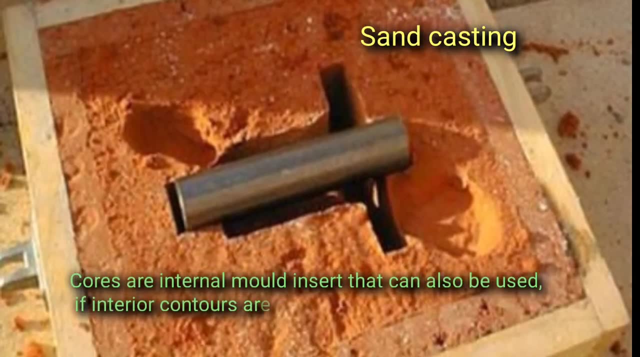 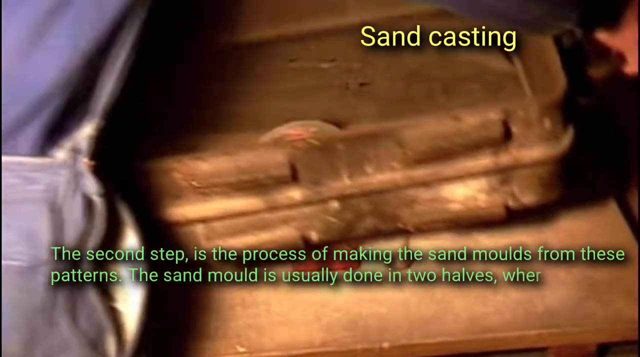 patterns are often made from materials such as wood, plastics etc. and are oversized to allow the cast metal to shrink. when cooling Cores are internal mold insert, that can also be used if interior contours are needed. The second step is the process of making the sand mold from this. 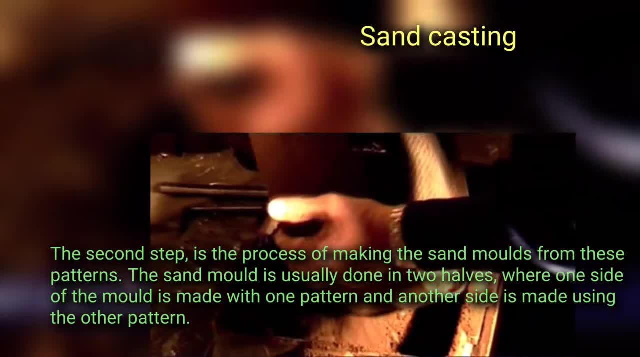 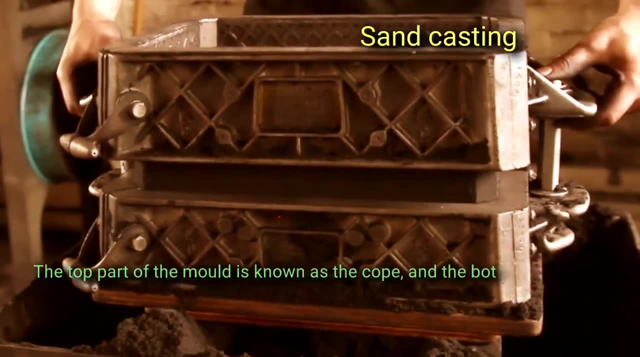 pattern. The sand mold is usually done in two halves, where one side of the mold is made with one pattern and the other side of the mold is made with another pattern. The sand mold is usually made with one pattern and another side is made using the other pattern. The top part of the 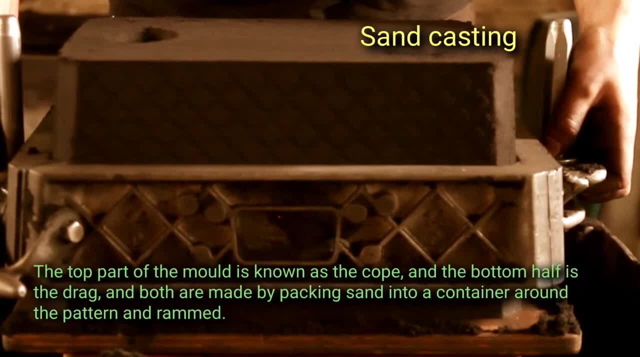 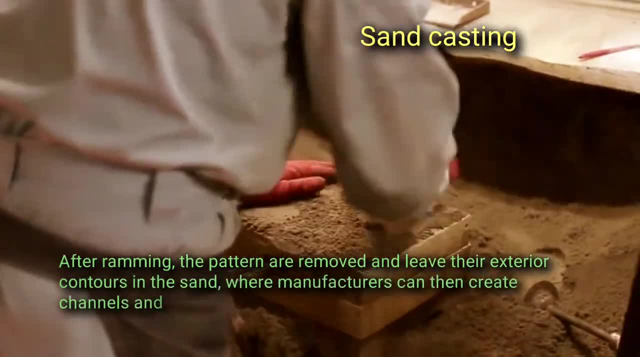 mold is known as the cope and the bottom half is the drag, And both are made by packing sand into a container around the pattern and rammed. After ramming, the pattern are removed and leave their exterior contours in the sand, where manufacturers can then create channels and connections. 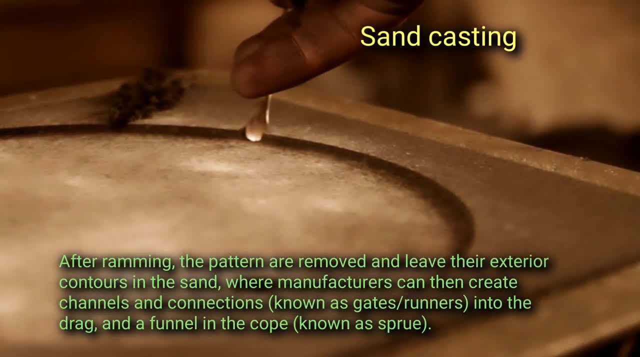 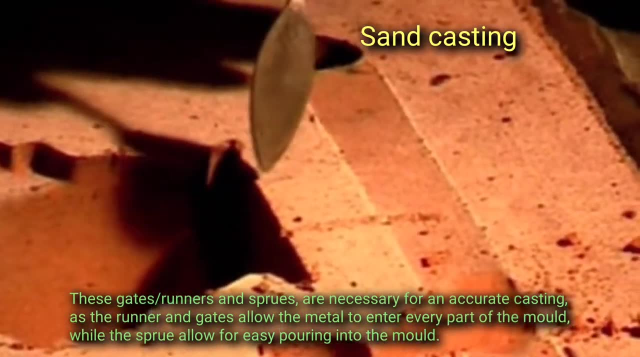 known as gates, runners into the drag and a funnel in the cope known as sprue. This gate runners and sprue are necessary for an accurate casting, as the runner and gate allows the metal to enter every part of the mold. 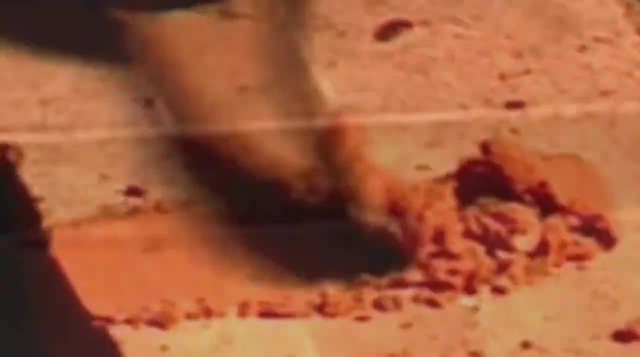 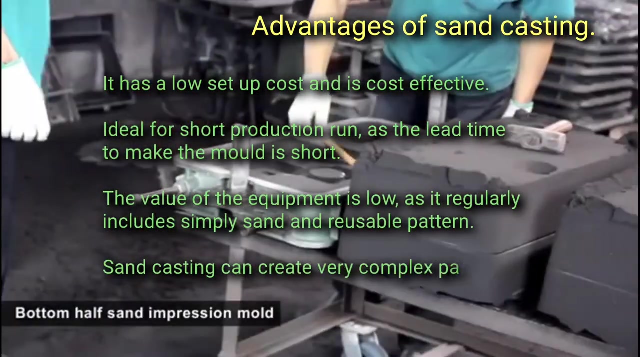 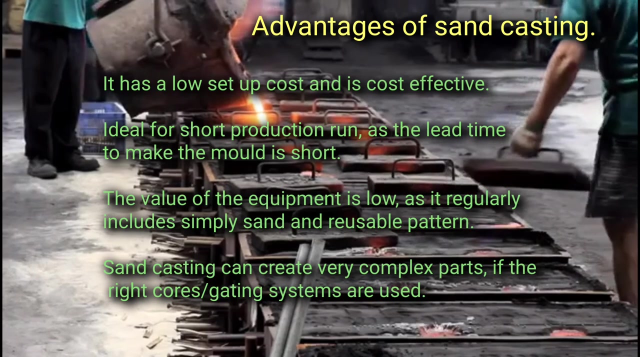 the sprue allow for easy pouring into the mold. Advantages of sand casting: It has a low set up cost and is cost effective. Ideal for short production runs as the lead time to make the mold is short. The value of the equipment is low as it regularly includes simply sand and reusable pattern. 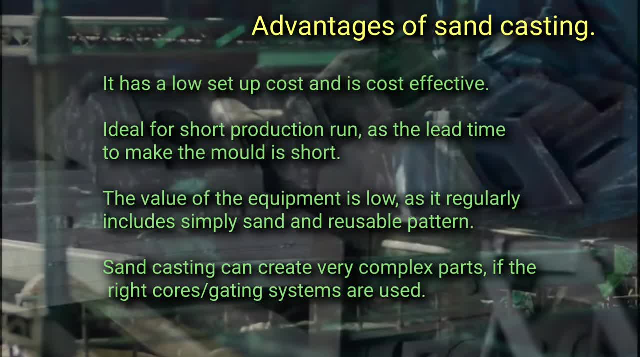 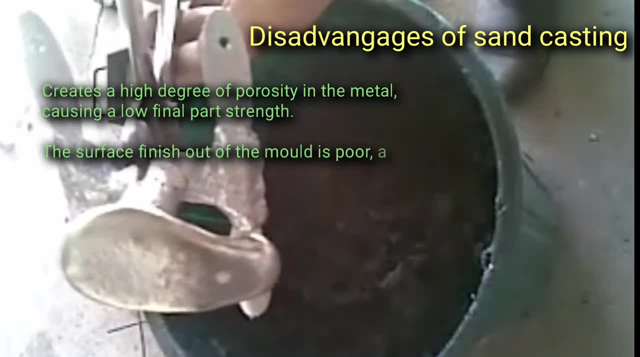 Sand casting can create very complex parts if the right cores and gating system are used. Disadvantages of sand casting Creates a high degree of porosity in the metal, causing a low final part strength. The surface finish out of the mold is 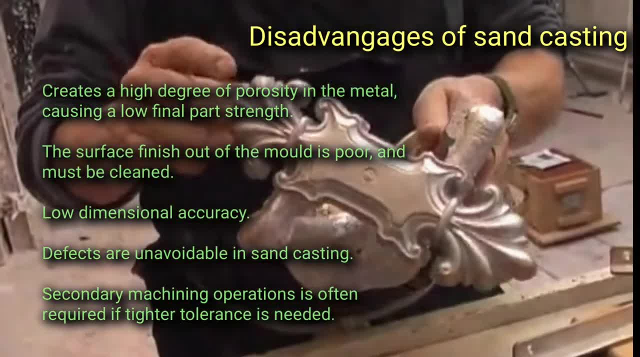 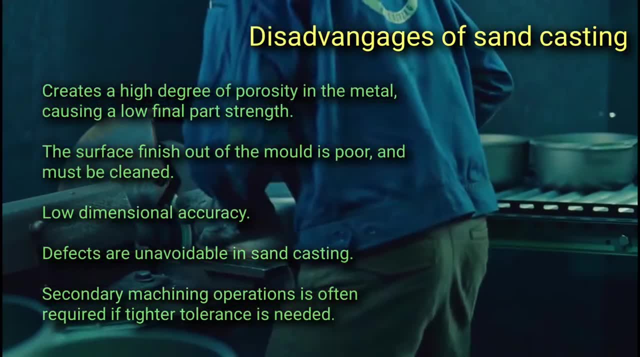 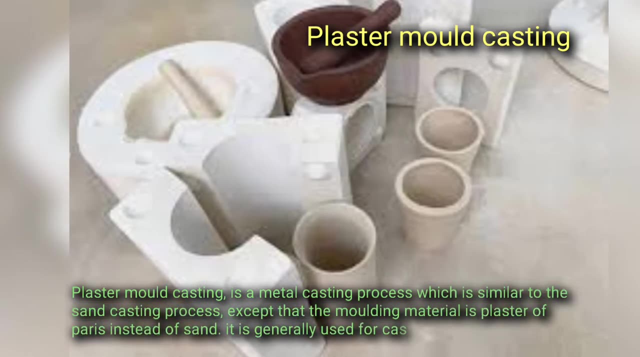 poor and must be cleaned. Low dimensional accuracy Defects are unavoidable in sand casting. Secondary machining operations is often required if tighter tolerance is needed. Plaster mold casting. Plaster mold casting is a metal casting process which is similar to the sand casting process. 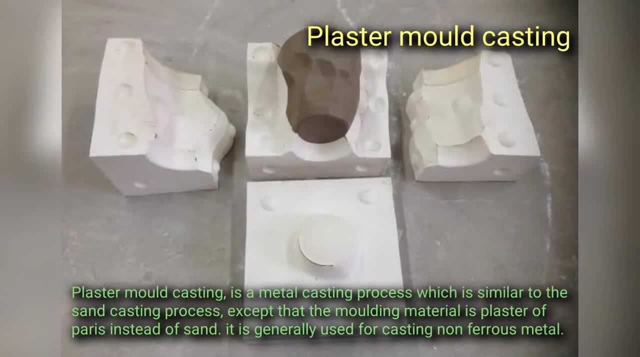 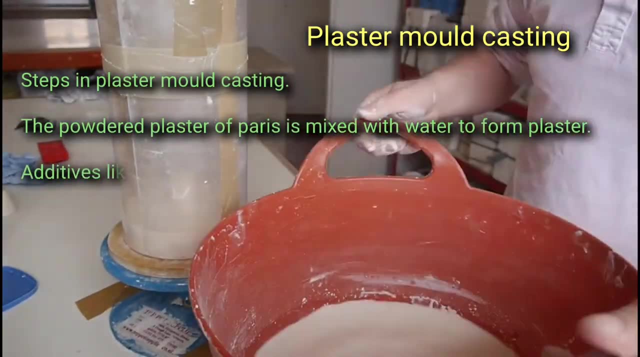 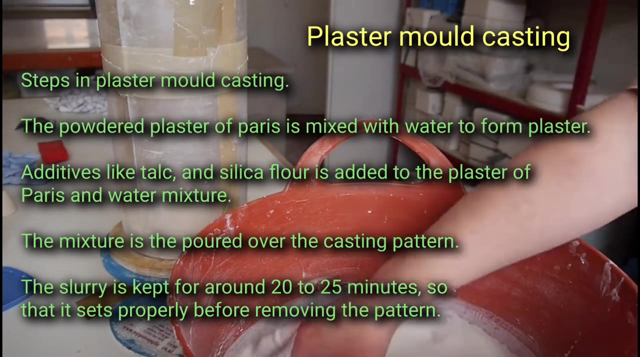 except that the molding material is plaster of paris instead of sand. it is generally used for casting. non-ferrous metals steps in plaster mold casting. the powdered plaster of paris is mixed with water to form plaster. additives like talc and silica flour is added to the plaster of paris. 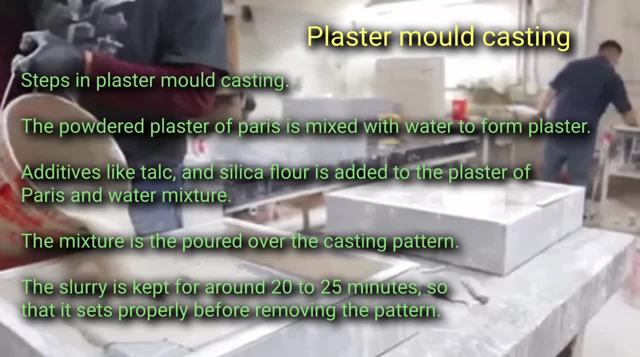 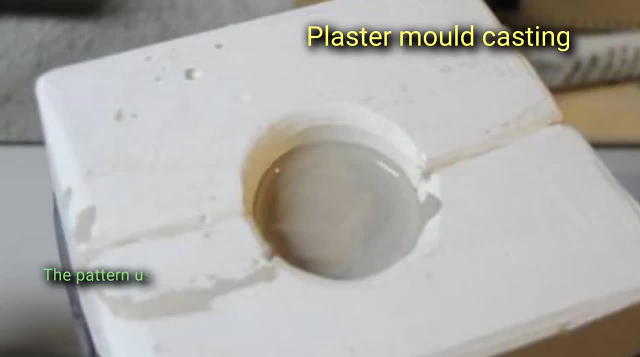 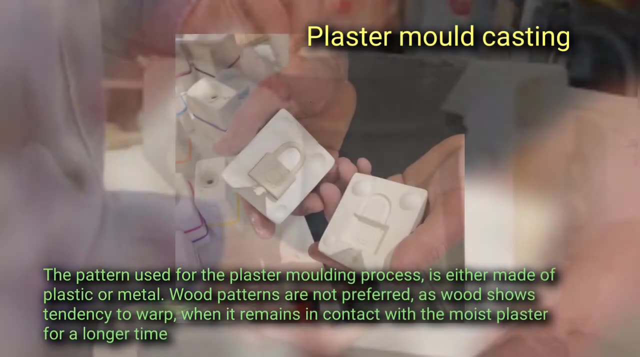 and water mixture. the mixture is then poured over the casting pattern. the slurry is kept for around 20 to 25 minutes so that it sets properly before removing the pattern. the pattern used for the plaster molding process is either made of plastic or metal. wood patterns are not preferred as wood. 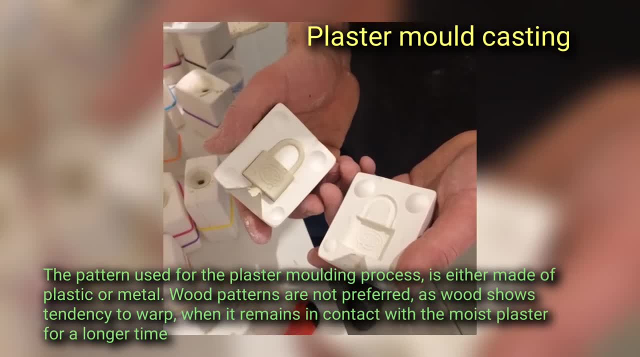 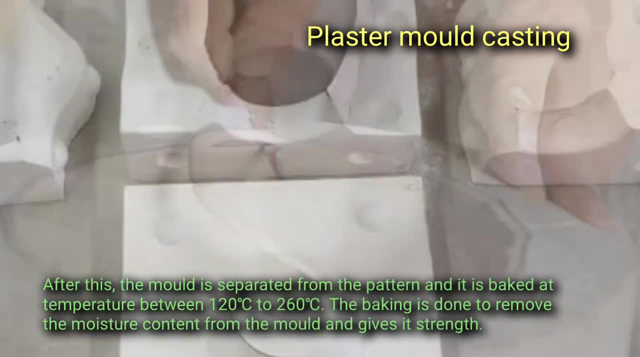 shows tendency to warp when it remains in contact with the moist plaster for a longer time. after this, the mold is separated from the pattern and it is baked at temperature between 120 to 260 degree celsius. the baking is done to remove the moisture content from the 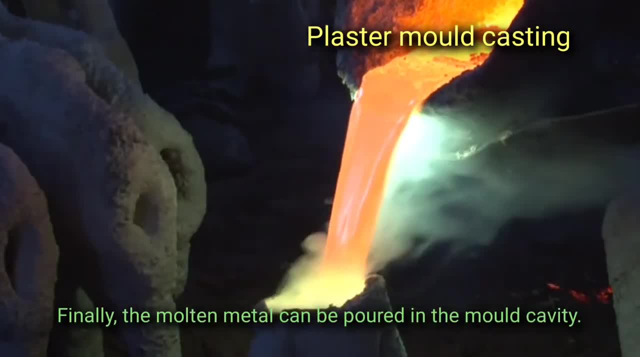 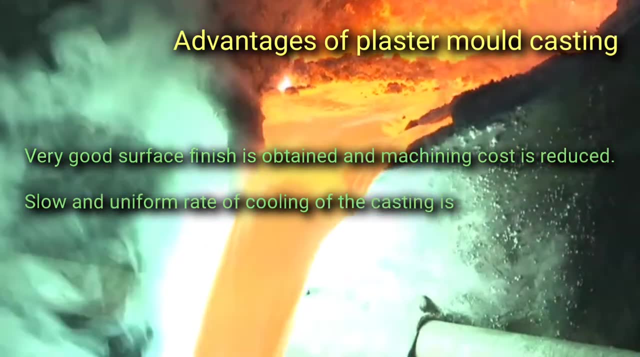 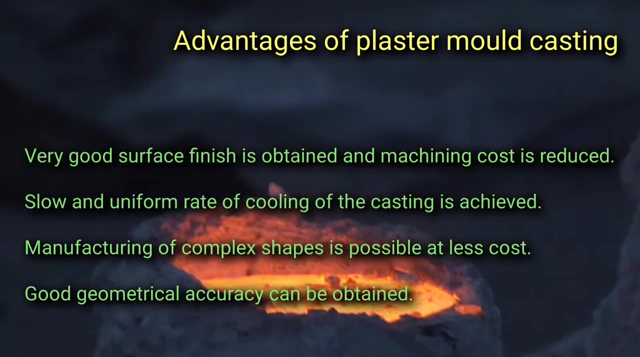 molding material and the plaster molding process is then made of plastic or metal. wood patterns mold and gives it strength. finally, the molten metal can be poured in the mold cavity. advantages of plaster mold casting: very good surface finish is obtained and machining cost is reduced. slow and uniform rate of cooling of the cast is achieved. manufacturing of complex 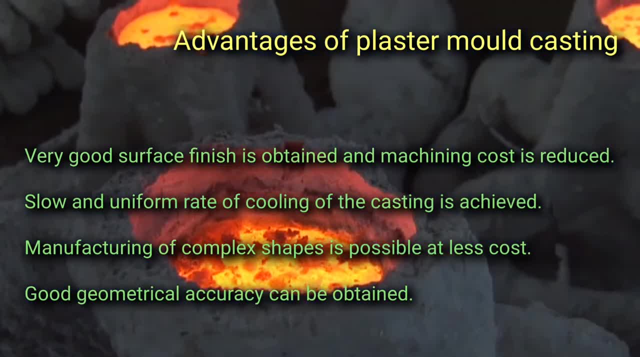 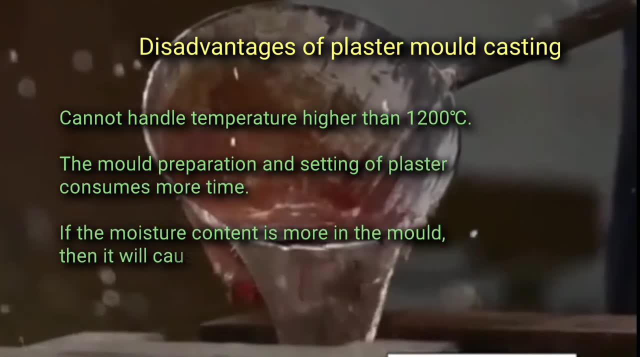 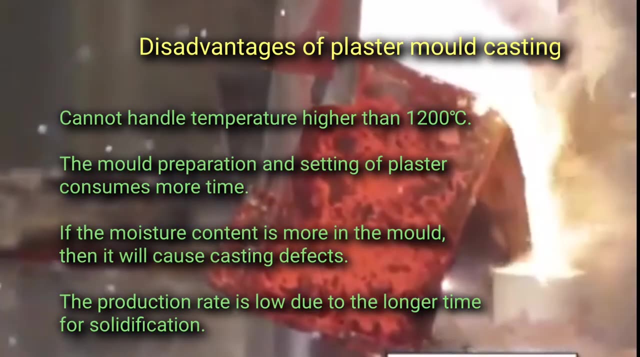 shapes is possible at less cost. good geometric accuracy can be obtained. disadvantages of plaster: mold casting cannot handle temperature higher than 1200 degree celsius. the mold preparation and setting of plaster consumes more time. if the moisture content is more in the mold, then it will cause casting defects. the production rate is low due to the longer time for solidification. 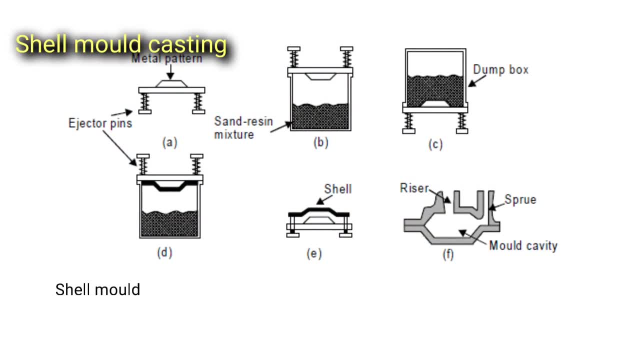 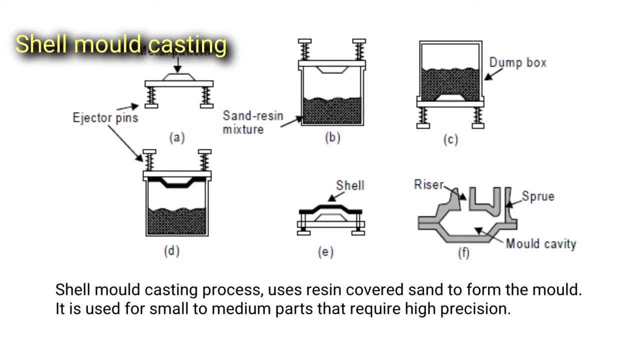 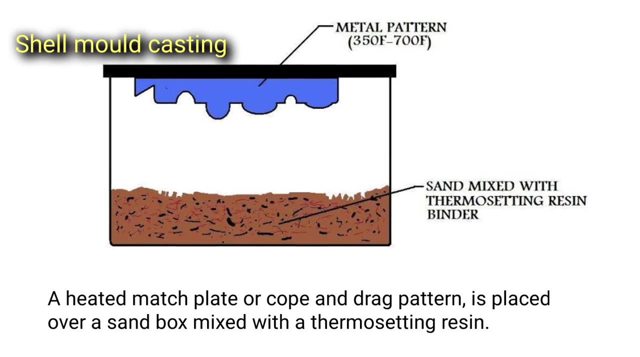 shell mold casting. shell mold casting process uses resin covered sand to form the mold it is used for small to medium part require high precision steps. in shell mold casting, a heated mach plate or cope and drag pattern is placed over a sand burden and can move with the help of tape after filling the mold 대%. 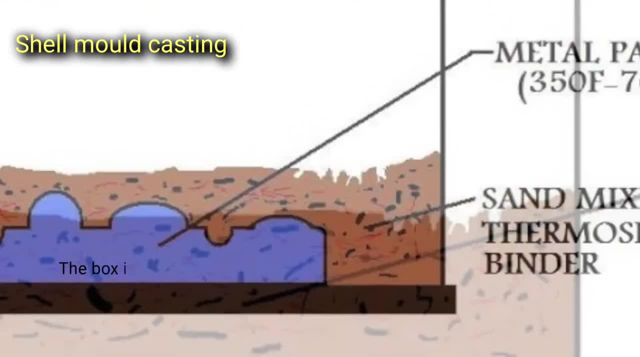 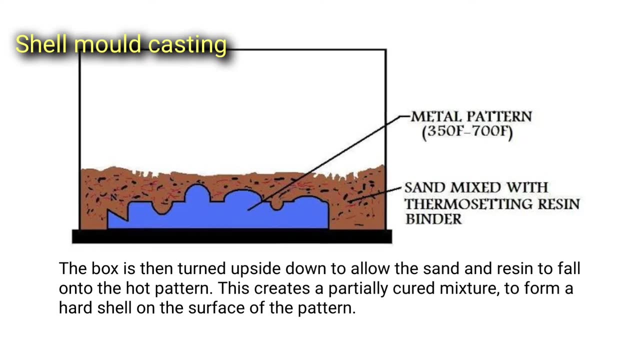 over a sandbox mixed with a thermosetting resins. The box is then turned upside down to allow the sand and resin to fall onto the hot pattern. This creates a partially cured mixture to form a hard steel on the surface of the pattern. The sand shell is cured by. 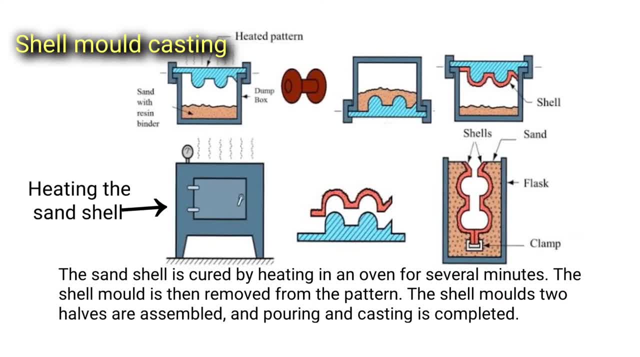 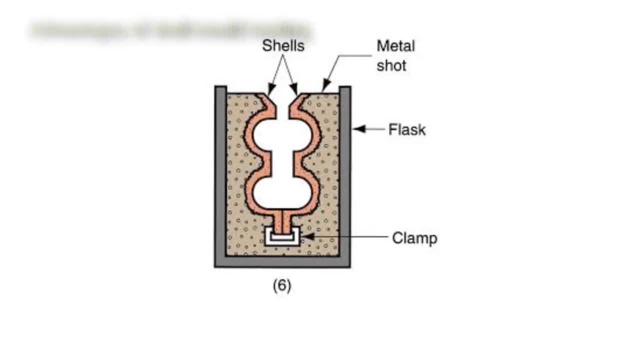 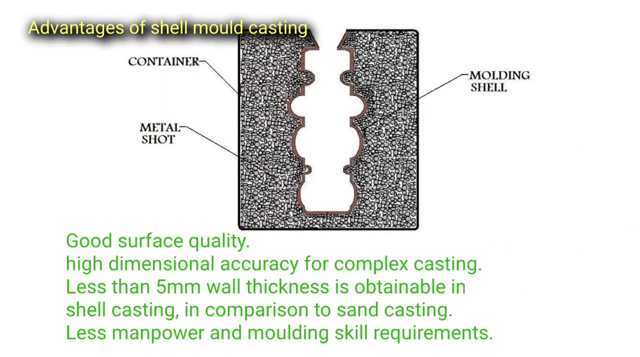 heating in an oven for several minutes. The shell mold is then removed from the pattern. The shell molds, two halves are assembled, and pouring and casting is completed. Disadvantages of shell mold casting: Good surface quality. High dimensional accuracy for complex casting. Less than 5mm wall thickness is obtainable in shell casting. in comparison, 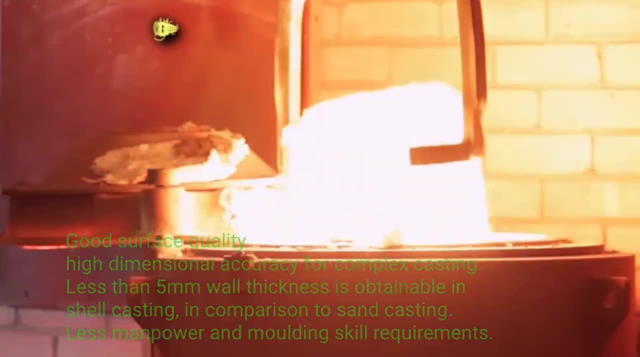 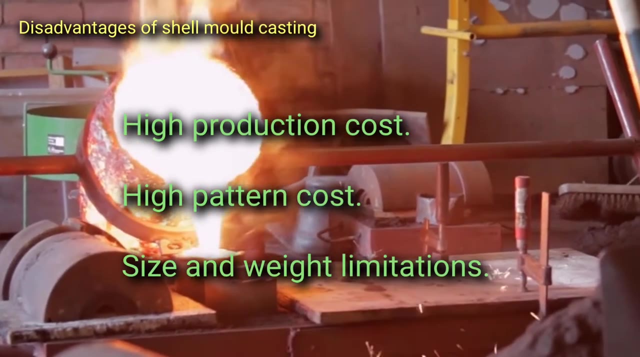 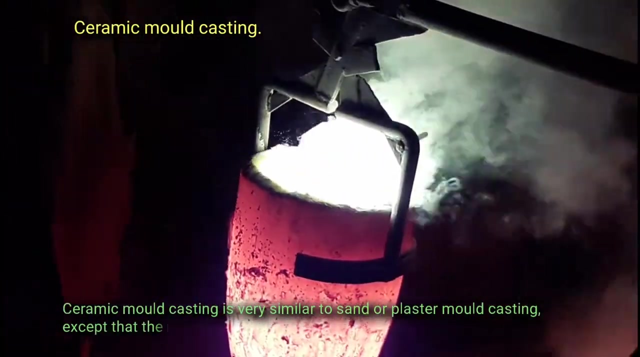 to sand casting: Less manpower and molding skill requirements. Disadvantages of shell mold casting: High production cost, High pattern cost, Size and weight limitations. Ceramics mold casting. Ceramics mold casting is very similar to sand or plaster molding. Ceramics mold casting has a lot of different. 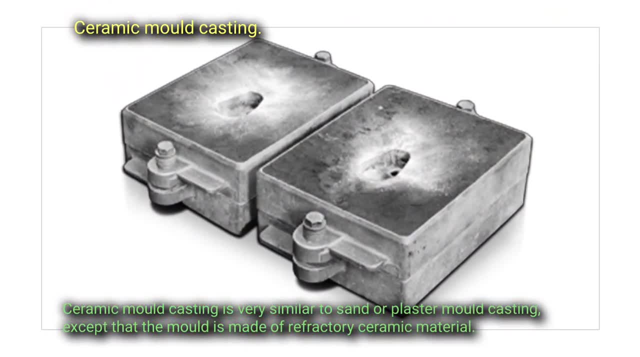 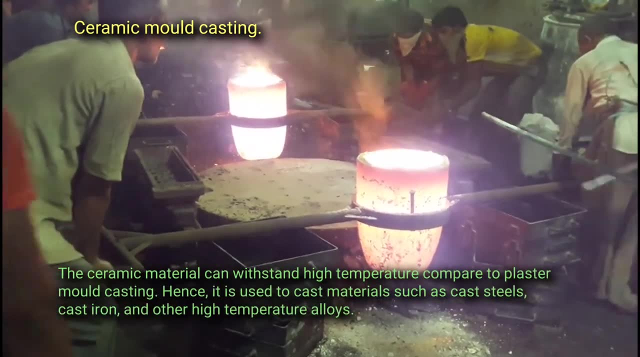 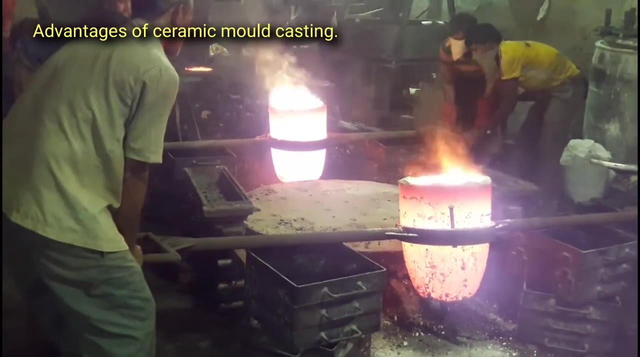 mold casting, except that the mold is made of refractory ceramic material. the ceramic material can withstand high temperature compared to plaster mold, hence it is used to cast materials such as cast steels, cast iron and other high temperature alloys. advantages of ceramics mold casting: excellent surface finish, closed dimensional tolerance, thin, cross-section and intricate. 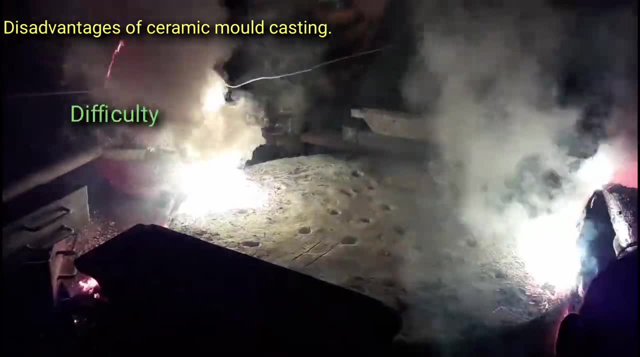 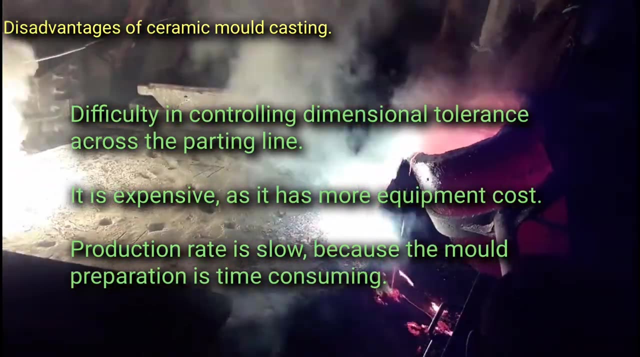 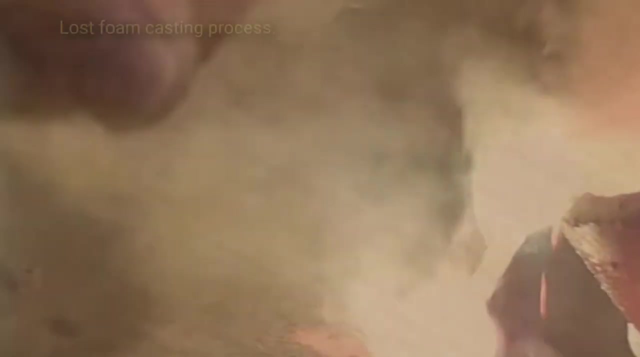 shapes can be cast. disadvantages of ceramics: mold casting. difficulty in controlling dimensional tolerance across the parting lines. it is expensive as it has more equipment. cost production rate is slow because the mold preparation is time-consuming. lost foam casting. lost foam casting is a type of evaporative pattern casting. this method is 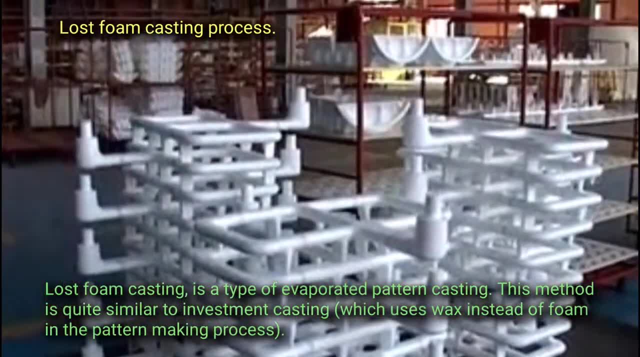 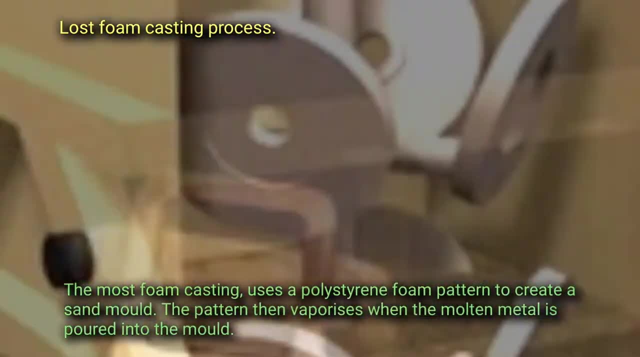 quite similar to investment casting, which uses wax instead of foam in the pattern making process. the lost foam casting uses a polystyrene foam pattern to create either Sandmole. the pattern vaporizes when the molten metal is poured into the mold it is sometimes referred to. 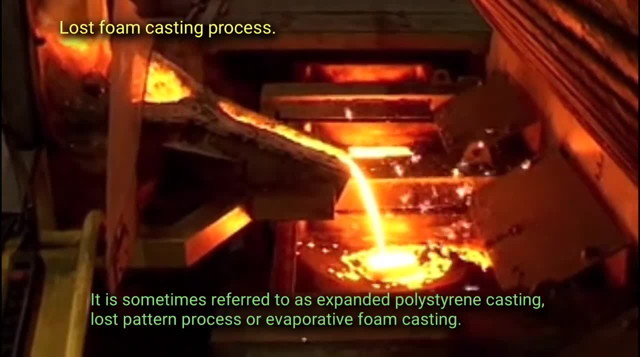 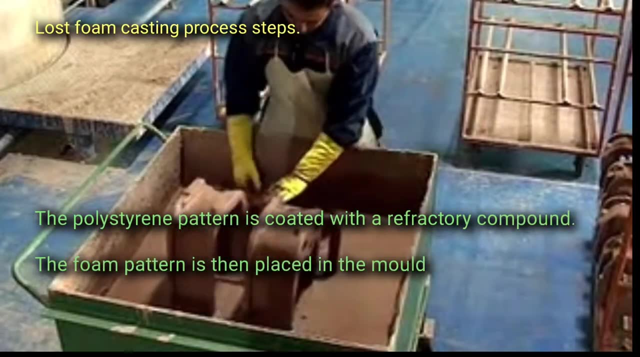 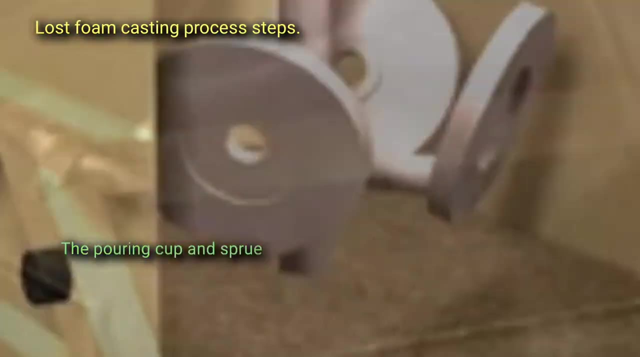 as expanded polystyrene, costing lost pattern. processor of operative foam casting. last foam casting process steps: the polystyrene pattern is coated with a refractory compound. the foam pattern is then placed in the mold box and spanned is compacted around it. the pouring 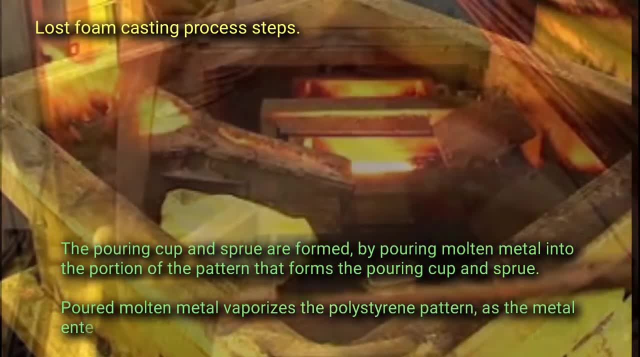 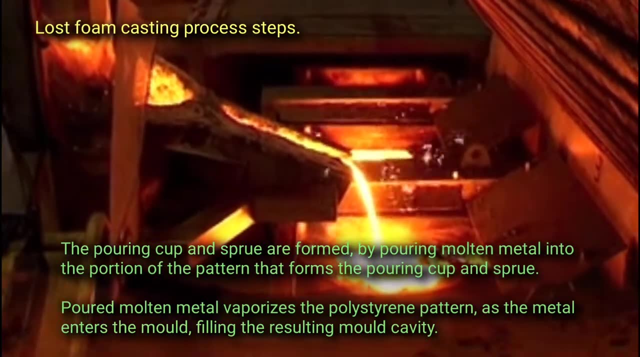 and sprues of the passive foam casting. the foam casting process steps: the soaps are formed by pouring molten metal into the portion of the pattern that forms the pouring cup and sprue. poured molten metal vaporizes the polystyrene pattern as the metal enters the mold filling. 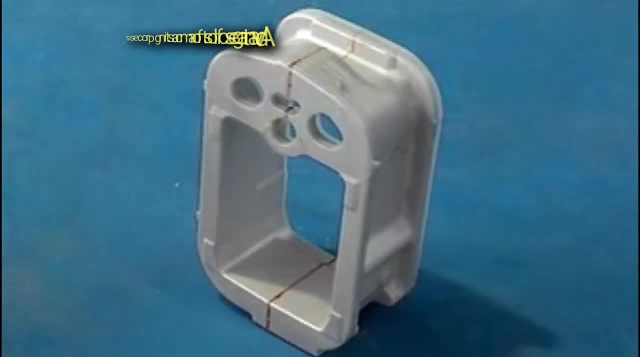 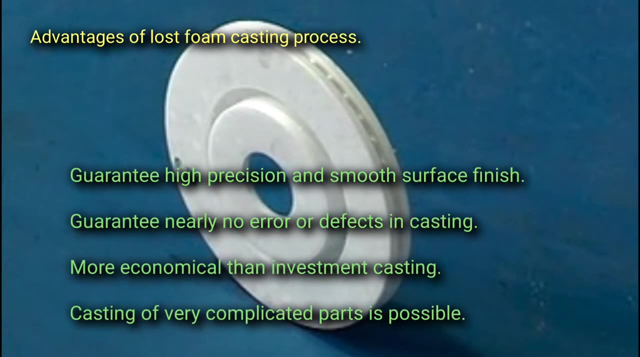 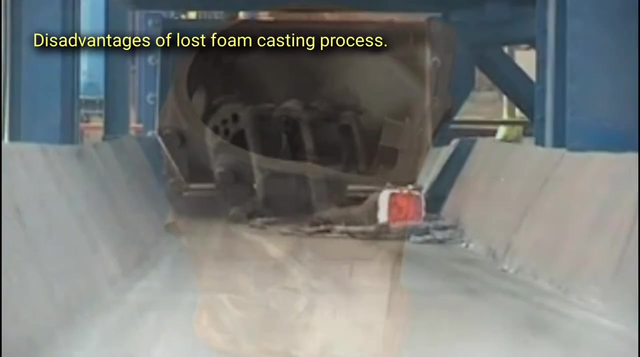 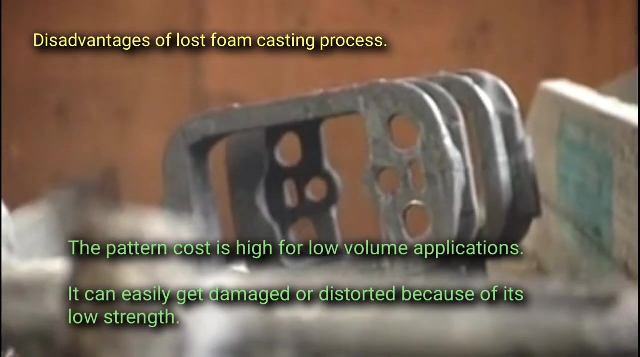 the resulting mold cavity. advantages of lost foam casting: guarantee high precision and smooth surface finish. guarantee nearly no error or defects in casting. more economical than investment casting. casting of very complicated parts is possible. disadvantages of lost foam casting: the pattern cost is high for low volume applications. it can easily get damaged or distorted because 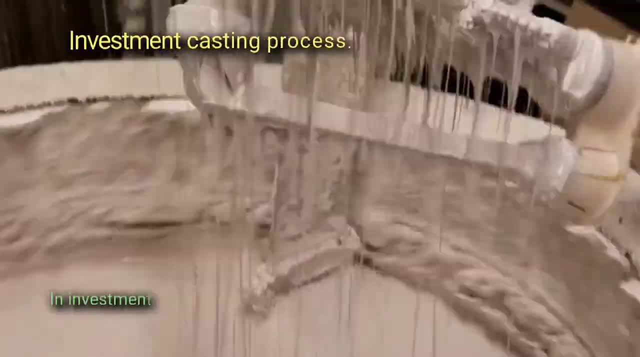 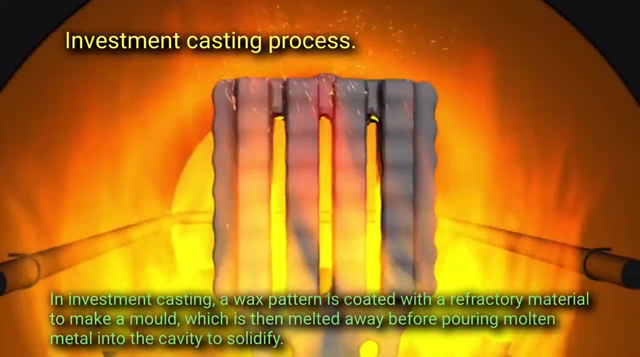 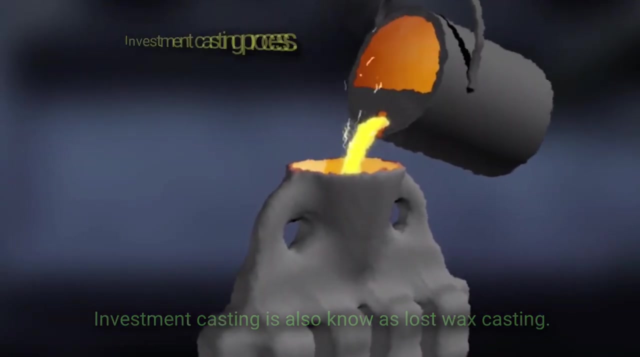 of its low strength investment casting process. in investment casting, a wax pattern is coated with a refractory material to make a mold which is then melted away before pouring molten metal into the cavity to solidify. investment casting is also known as lost wax casting. advantages of investment casting: parts with extremely complex shapes and intricate feature. 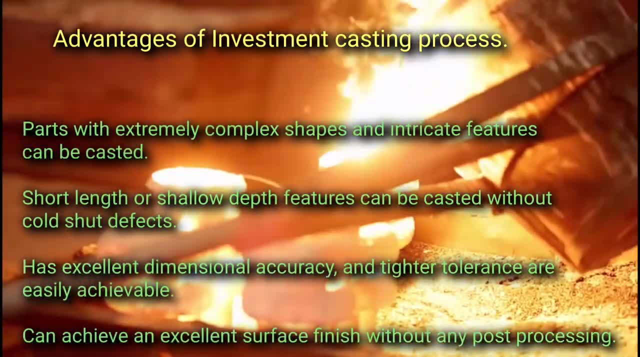 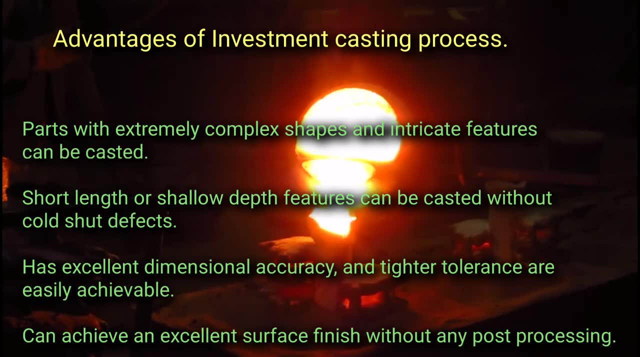 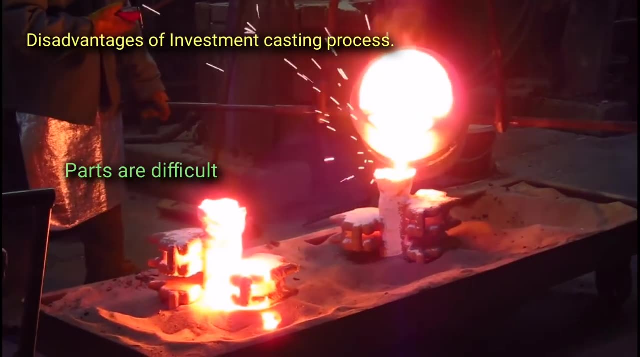 can be casted as a single piece. short length or shallow depth features. can be casted without cold shut defects. has excellent dimensional accuracy and tighter tolerance, so easily achievable. can achieve an excellent surface finish without any post-processing disadvantages of investment. casting parts are difficult to cast if they require core limited to large production qualities. 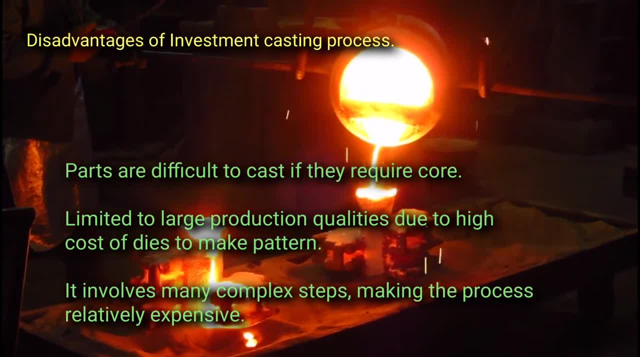 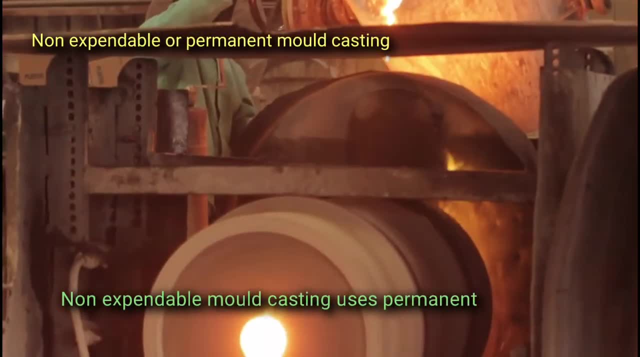 due to high cost of dust. disadvantages of investment. casting parts are difficult to cast if they require core. limited to large production qualities due to high cost of dust. due to high cost of dust dies. to make patterns. it involves many complex steps, making the process relatively expensive. non-expendable or permanent mold casting. non-expendable mold casting uses permanent molds. 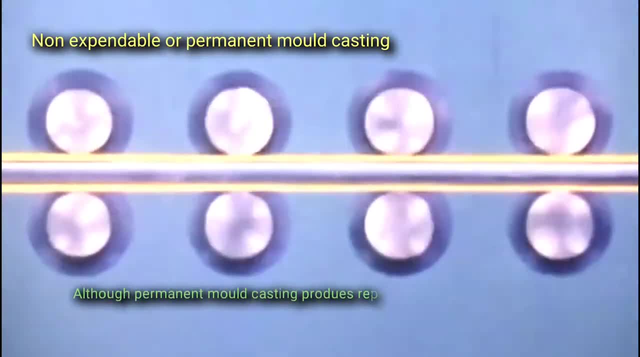 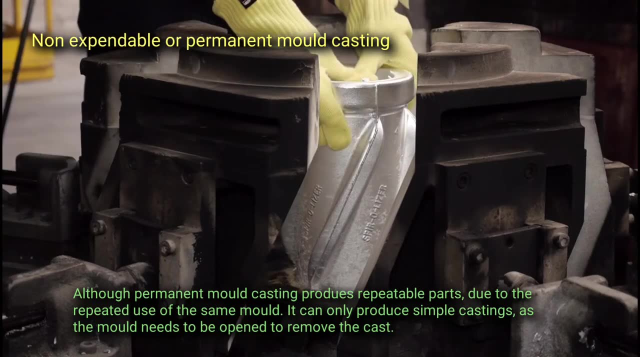 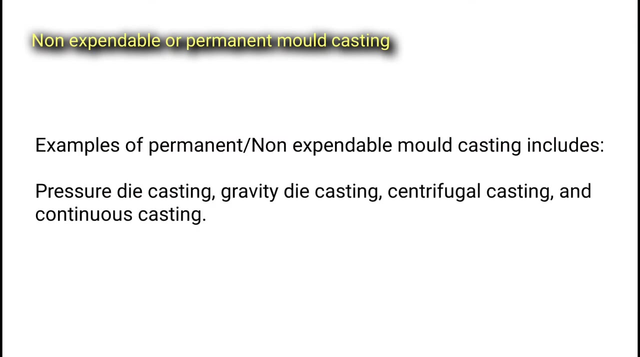 which can be reused after each production cycle. although permanent mold casting produces repeatable parts due to the repeated use of the same mold, it can only produce simple casting, as the mold needs to be open to remove the cast. examples of permanent mold casting includes pressure die casting, gravity die casting, centrifugal casting and continuous casting. 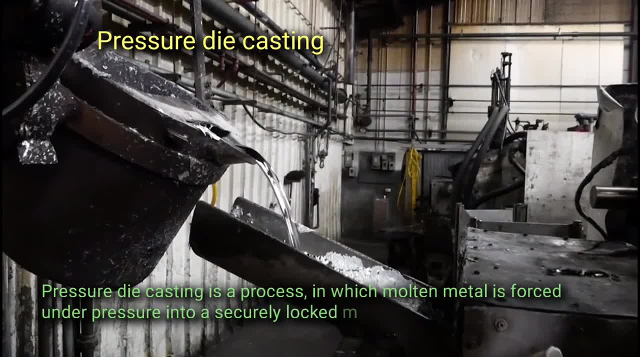 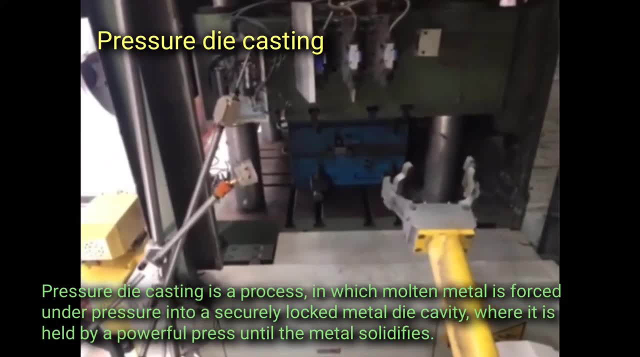 pressure die casting. pressure die casting is a process in which molten metal is forced under pressure into a securely locked metal die cavity, where it is held by a powerful press until the metal solidifies. after solidification of the metal, the die is unlocked, opened and the contraлан surface of the——————ó–that—¡­s— Pepperoni——oleemail clay Detailed supporting sheet metal. die casting application had been completed at the Cosden Hall North. Issuares Horseman härtöru ב� geek führenø alü reg gearsä vocês¡�בא why–. 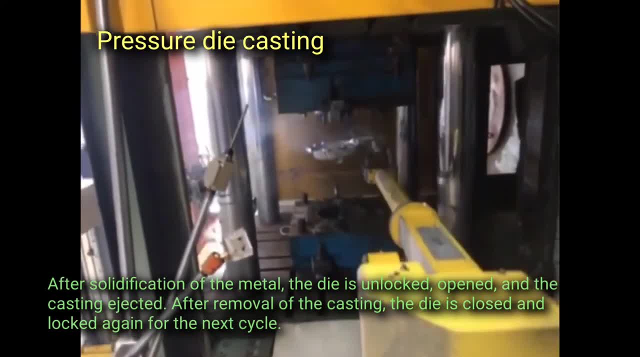 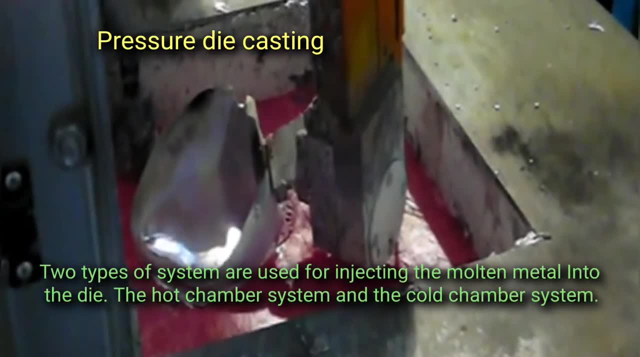 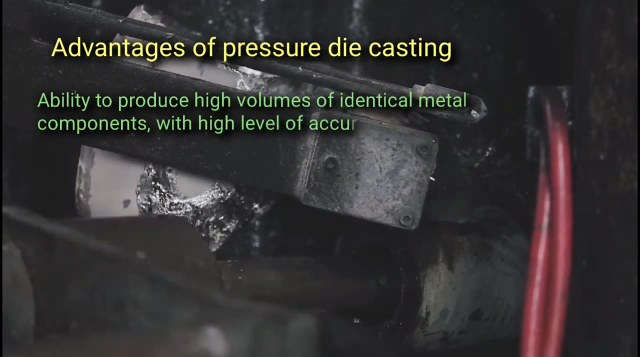 Casting ejected. After removal of the casting, the die is closed and locked again for the next cycle. Two types of system are used for injecting the molten metal into the die: The hot chamber system and the cold chamber system. Advantages of pressure die casting: Ability to produce high 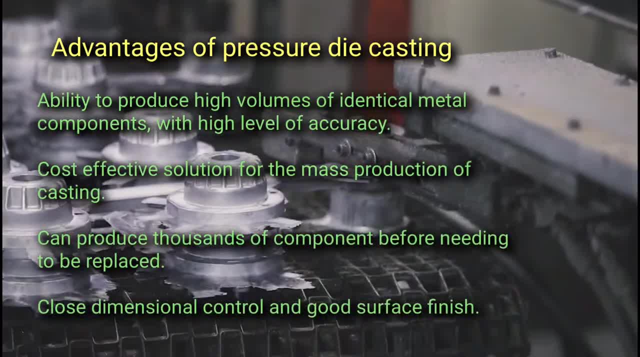 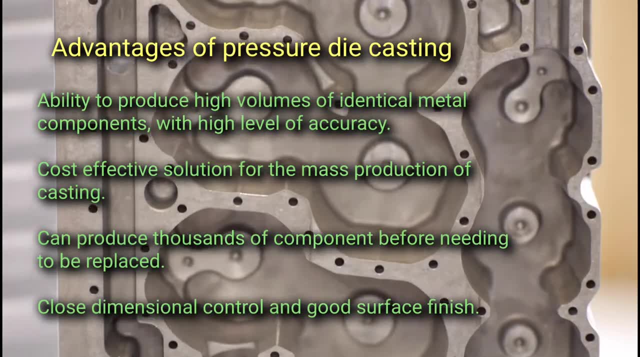 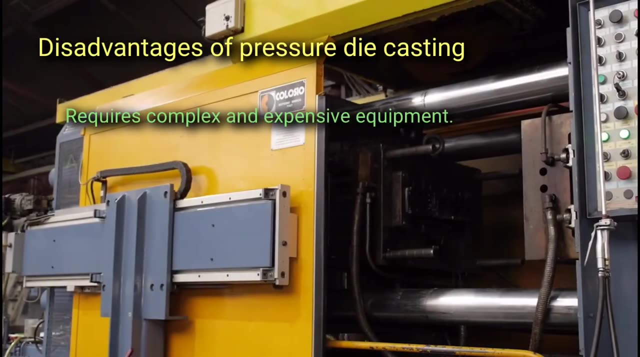 volumes of identical metal components with high level of accuracy. Cost effective solution for the mass production of castings can produce thousands of component before needing to be replaced. Close dimensional control and good surface finish. Disadvantages of pressure die casting Requires complex and expensive equipment. A large capital investment is required for the setup. 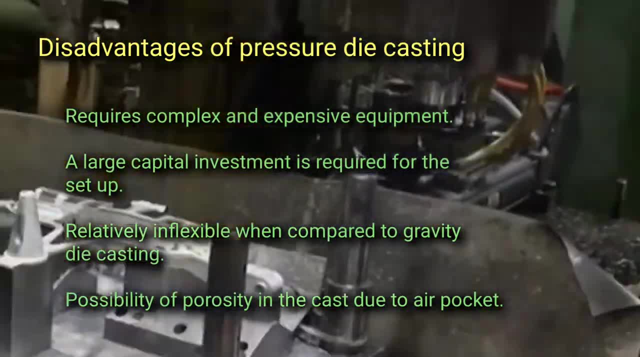 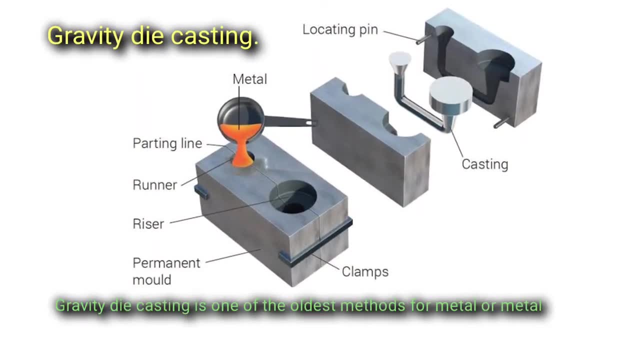 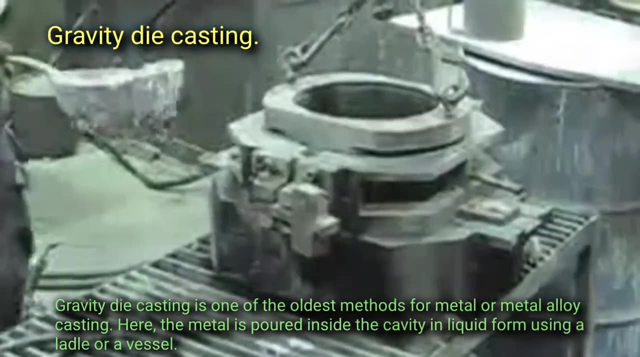 Relatively inflexible when compared to gravity die casting. Possibility of porosity in the cast due to air pockets. Gravity die casting- Gravity die casting is one of the oldest methods for metal or metal alloy casting. Here the metal is poured inside the cavity. 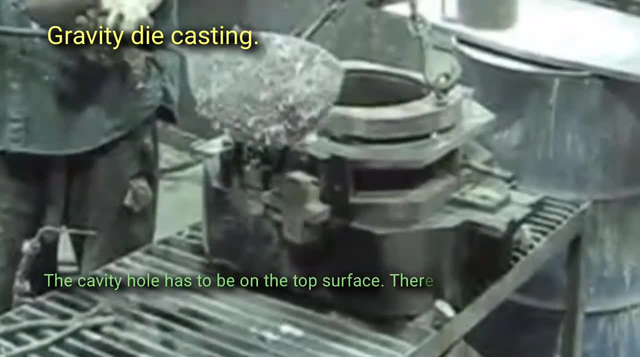 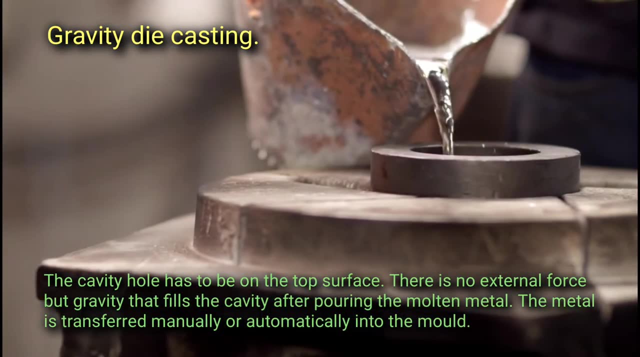 in liquid form using a ladle or a vessel. The cavity hole has to be on the top surface. There is no external force but gravity that fills the cavity. after pouring the molten metal, The metal is transferred manually or automatically into the mold. Sometimes it is necessary to tilt. 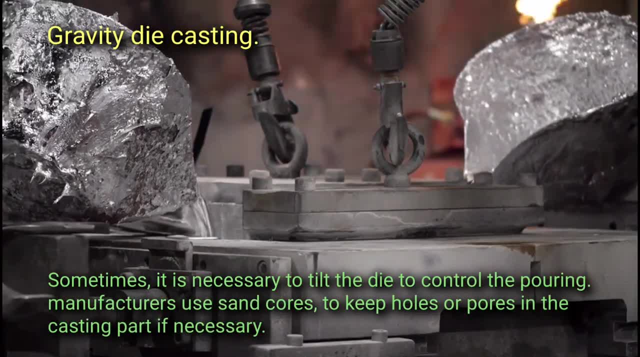 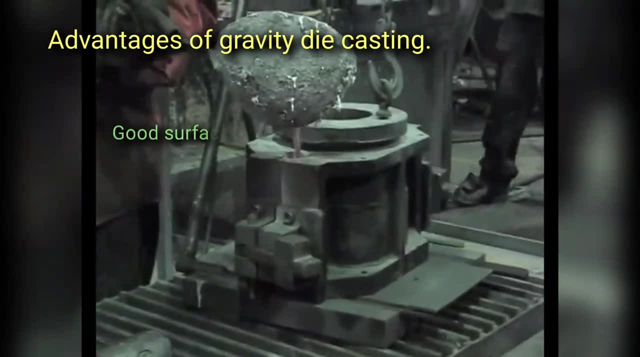 the die to control the pouring. Manufacturers use sand cores to keep holes or pores in the casting part, if necessary. Advantages of gravity: die casting: Good surface finish. Tight dimensions of the die. Gravity die casting. Good surface finish: Good surface finish Good. 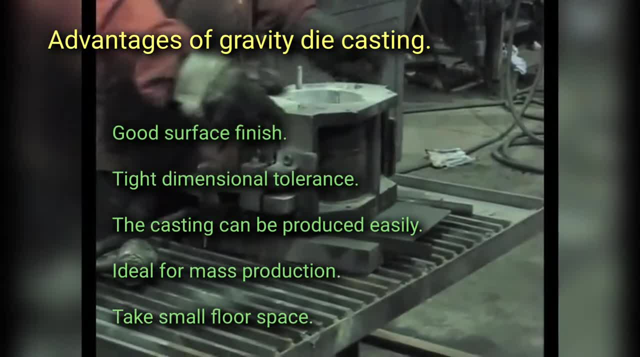 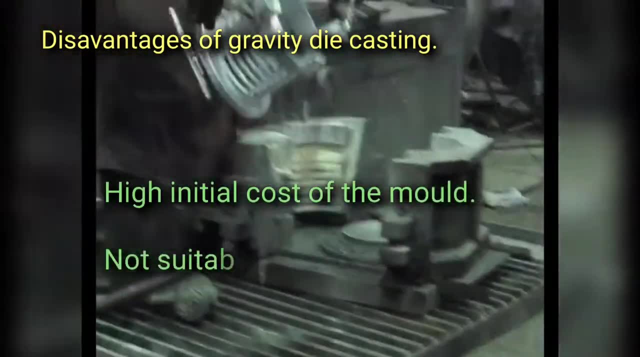 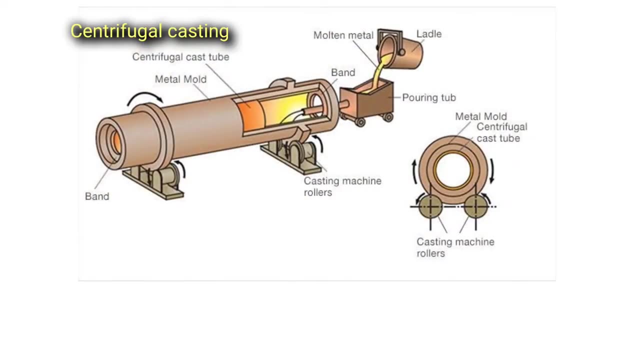 dimensional tolerance. Thin casting can be produce easily. Ideal for mass production: Take small floor space. Disadvantages of gravity: die casting. High initial cost of the mold. Not suitable for casting metals with a high melting point. Centrifugal casting: Centrifugal casting is a permanent molding process which makes use of 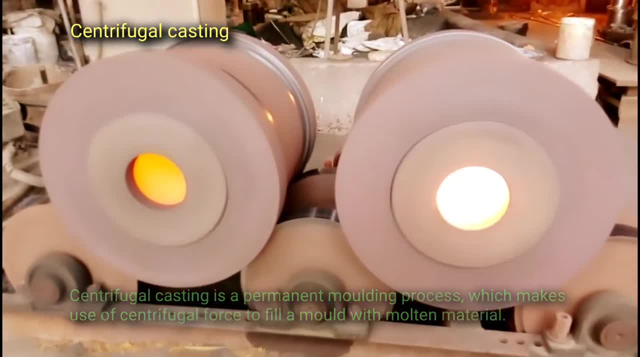 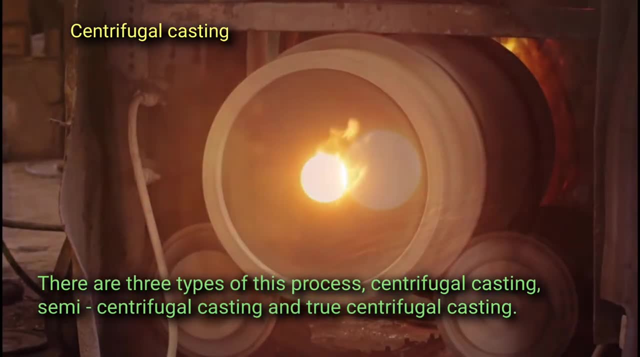 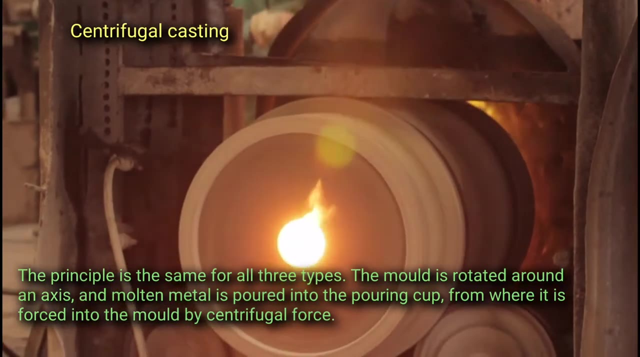 centrifugal force to fill a mold with molten material. There are three types of this process: Centrifugal casting, semi-centrifugal casting and true centrifugal casting. The principle is the same for all the three types: The mold is rotated around an axis and molten metal is poured into.